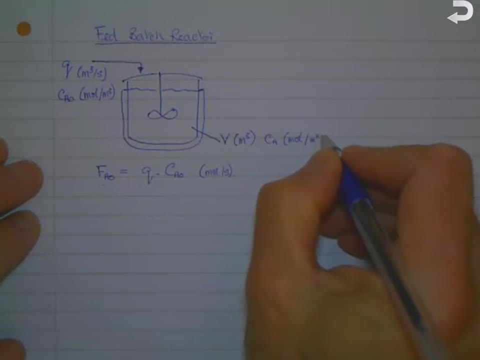 reactor of CA moles per cubic meter. once again, we can just use that relationship to derive the number of moles. so the number of moles of a at any given time is equal to the volume in the reactor multiplied by the concentration. that's just in moles. and I will define one other term, which is the reaction. 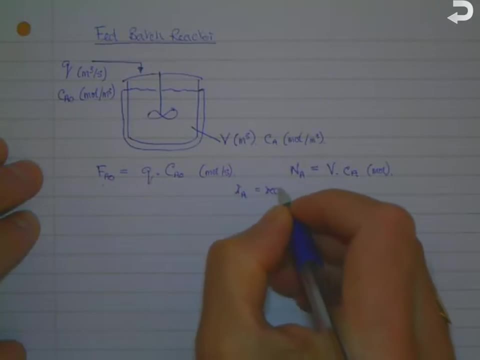 rate of a, that's RA, which is the reaction rate of a, and that if a is being consumed, as it is in our case, that will be a negative value because it's it's reacting away and being consumed for a product, it would be positive. so that's the reaction. 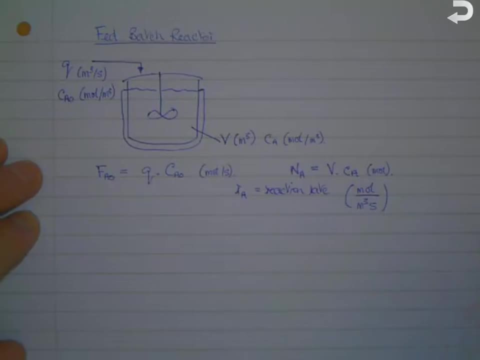 rate RA in moles per cubic meter per second. before we start, as always, we need to state the assumptions we're going to make. the first one is that the reactor is well mixed. what that means is that composition, temperature etc at any point in the reactor is the same as everywhere else and equal to the average. 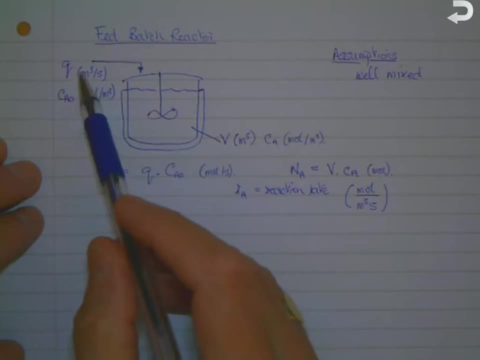 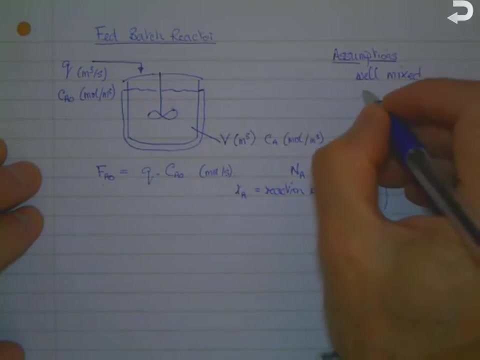 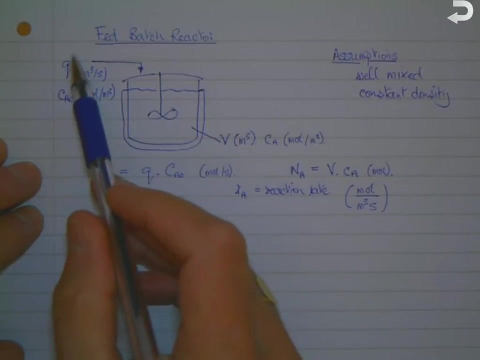 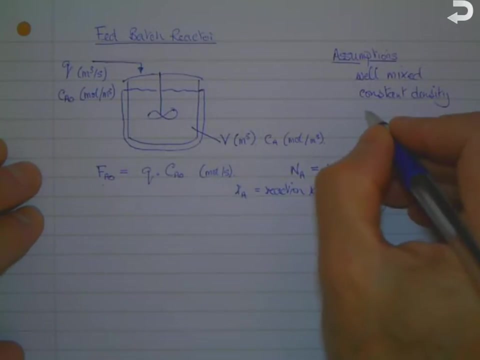 composition and that our added material Q is mixed in rapidly. we're also going to assume that we've got constant density, so that the density in the reactor is equal to the density of the added material and that that density doesn't vary with time over the time period of interest. and again for. 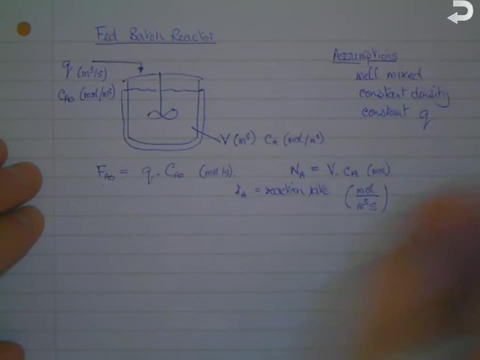 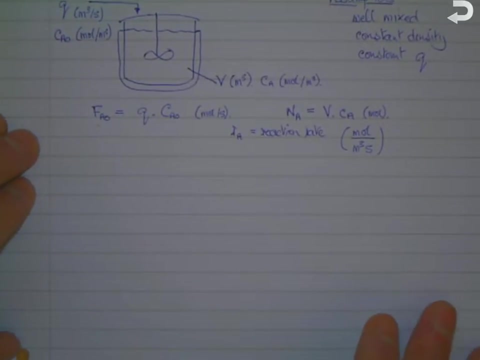 the sake of this derivation, we're going to assume that the addition rate Q is constant. okay, so to do the derivation, we do a material balance over a time interval of Delta T time interval, Delta T seconds, and we use the usual material balance equation, which is the input. 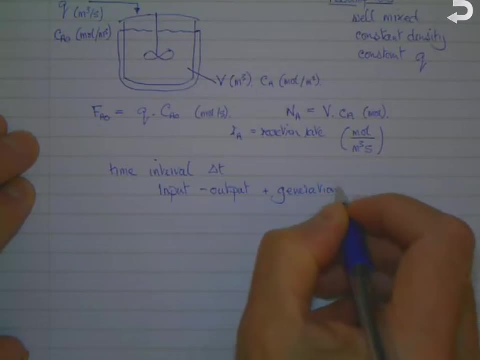 minus output, plus generation, equals accumulation. so in other words, what grows in and minus what goes out, plus any material which is generated by reaction, is equal to the, the build-up in the system, and then in this case we've got a batch process as a transient process, so we will have accumulation. 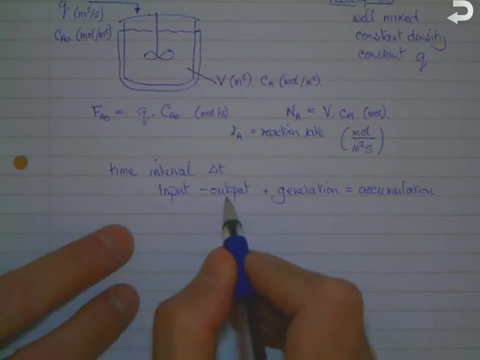 however, we don't have any output, that batch characterized by doing an addition with no removal of any material. so we can first of all do an overall material balance, an overall mass balance. but because we've got constant density we can effectively do a volumetric balance. so the input over Delta T is Q multiplied by Delta T. 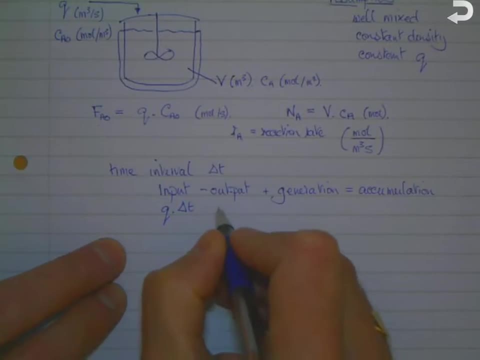 cubic meters being added, output is zero. we're not generating any mass. so overall there's no generation term for the overall balance and that equals the accumulation, and the accumulation is the volume at T plus Delta, T minus the volume that was there at the beginning of the time interval T, and we can just 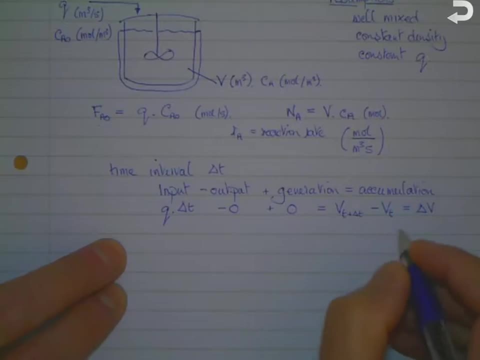 rewrite that as Delta V. so if we drop the zeros and collect the terms together, actually we can divide by Delta T. we can rewrite that as Q equals Delta V over Delta T, and as Delta T tends to zero, then we can replace that with the, with the derivative. so 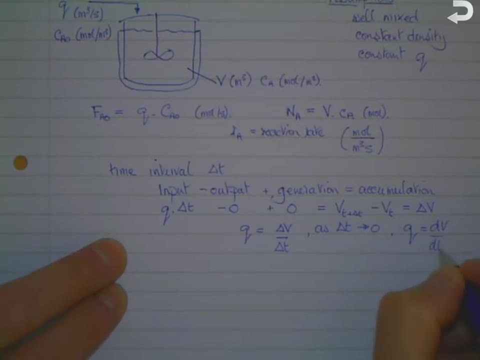 we can replace that with the with the derivative. so we can replace that with the with the derivative. so Q equals DV by DT and intuitively that makes sense. that's just saying that the, the rate of change of the volume in the in the reactor with time, is equal to the. 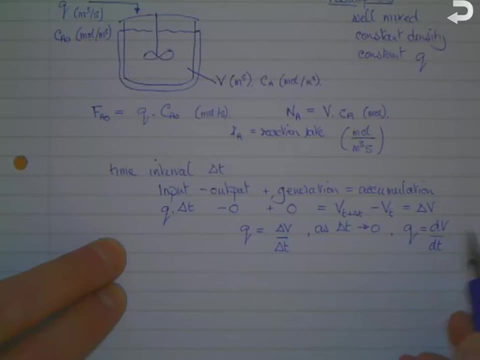 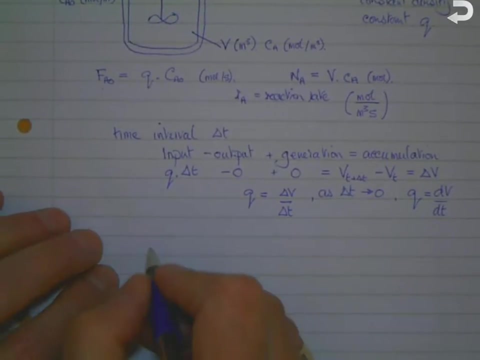 addition rate, and the addition rate is constant. so you've got a constant DV by DT, which is the same as the addition rate. okay, so now let's do the same thing for component a. so in this case we can say: over Delta T the input is equal to F a, not define that. 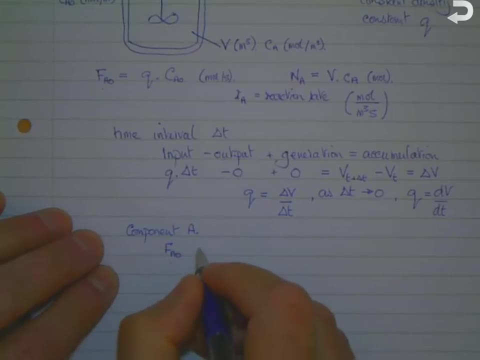 above, minus the output, which is zero, again plus generation. so we've got a reaction term, this this time because a is reacting away, so we can have our a, which is the reactor right. moles per cubic meter per second, so an to multiply by the volume V and by the time interval, Delta T and, of course, 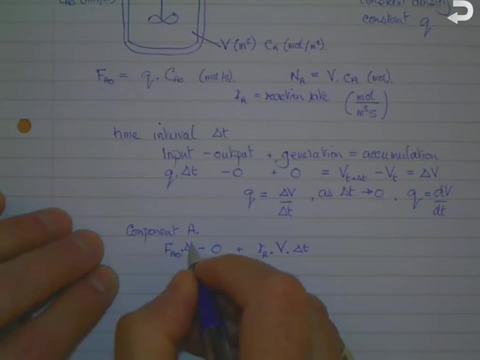 we've got to multiply our molar flow rate by Delta T as well. so we've got FA naught times Delta T, which is the number of moles added in time interval Delta T, and then we've got RA times V times Delta T, which is the number of. 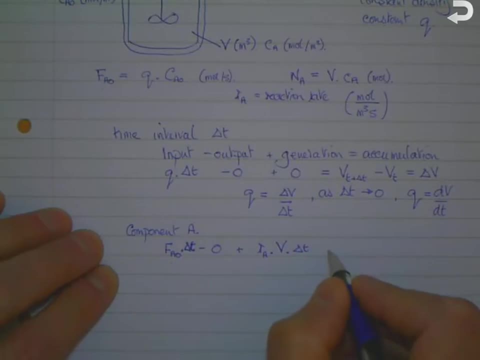 moles which have been consumed due to the reaction, and that's equal to an a at the end of our time interval, number of moles in the reactor minus the number of moles in the reactor at the beginning of our time interval, and a T, and that can: 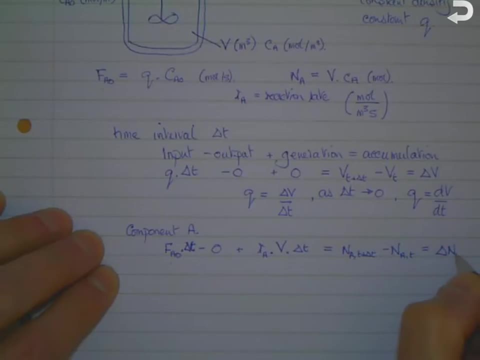 simply be written as n a, Delta n a. so if we now divide by Delta T, we get that FA naught plus RA times V is equal to Delta n a over Delta T, and as Delta T tends to 0, that becomes the derivative DNA by the T and we can. 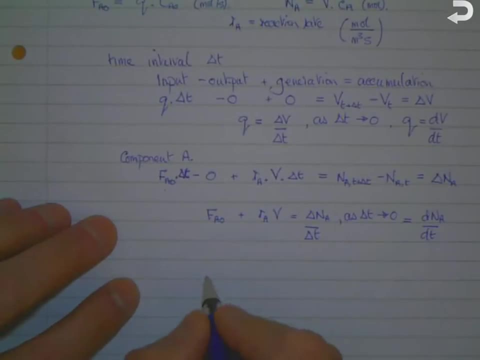 rewrite. rewrite that in terms of concentrations so we can replace Q. it could place FA naught by Q times CA naught. I have Q times CA naught plus RA times V equals D by DT. I'm going to replace an a by V times CA, so that's D by DT of V times CA. now both. 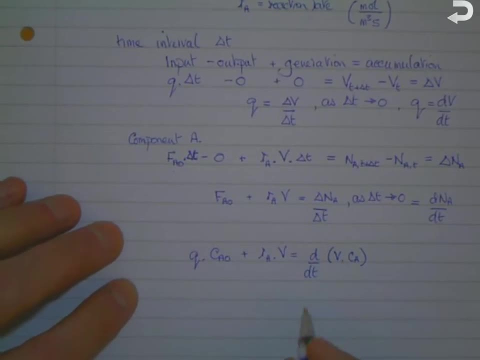 V and CA vary with time. so we've got the, the differential of a product there. so D of X times Y by DT is equal to X times dy by DT plus Y times the X by DT. so we can consume that and we get that C Q times CA naught plus RA times V naught. 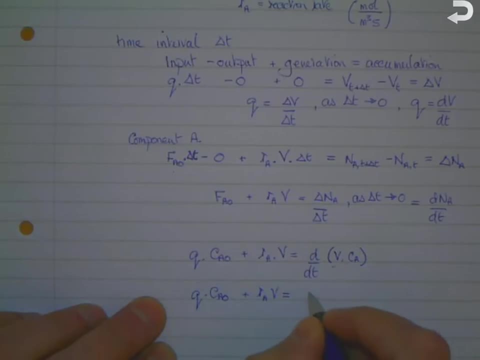 equal V by DT times VA by da. this would be V by DT. am I right? but I third, it can actually be cualit 단 equal T times DEV by DT. but DV by DT is equal to Q, so we can substitute in here: going to q is equal to K and ds by dt is. 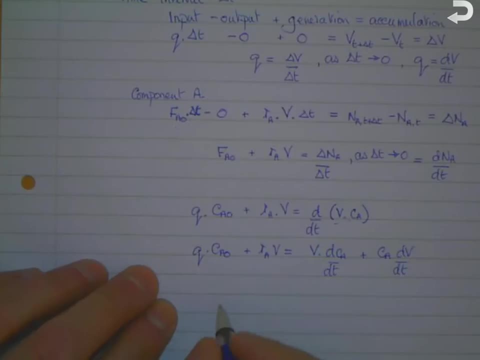 conjure up lots of titles we've got, so we put them together. so today going to do, ironically, we're going to give you a times CA0, so RA times V is equal to V DCA by DT plus Q times CA. And if we then divide,